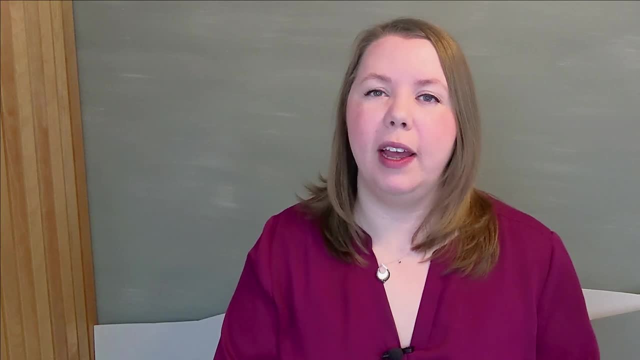 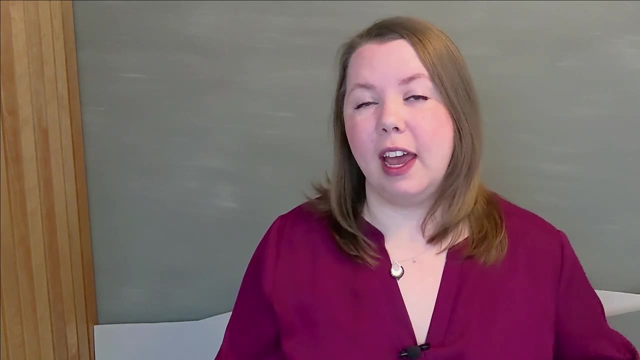 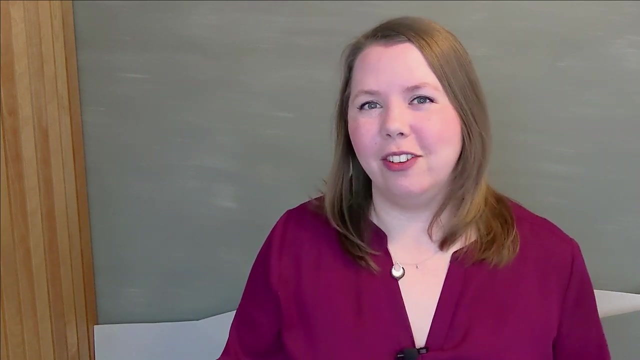 on a daily basis is that there's also a lot of healthcare data analysts employed by state and local governments, either in general statistics collection, like in the case of Statistics Canada, or in monitoring public health and the performance of different hospitals and providers, Because there isn't just one healthcare data analyst role. the day-to-day work for these 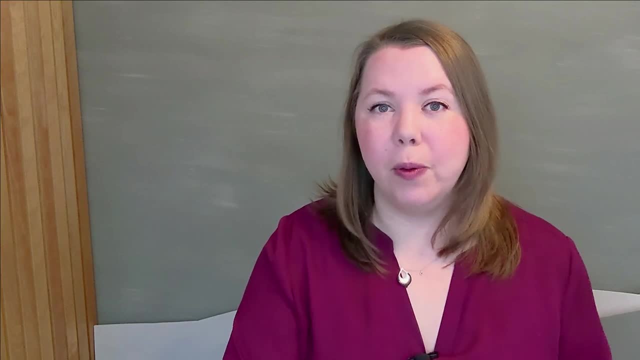 jobs can look a little different depending on who you're employed by and exactly what type of role you're looking at. Let's look at four broad categories that a healthcare data analyst can do on a daily basis. The first one is a healthcare data analyst. Healthcare data analysts are the ones that fall within the healthcare analytics field. There isn't a completely uniform application of titles across the roles, so keep in mind that jobs within each of these major areas may look slightly different from what I'm about to describe. But in general, these are four major categories where you'll find healthcare data analysts and the different specific things that they'll be working on. Let's start with healthcare data analysts working for healthcare providers. Healthcare providers range from primary care physicians to hospitals to even long-term care facilities. in general, these are roles that are very patient facing they're. 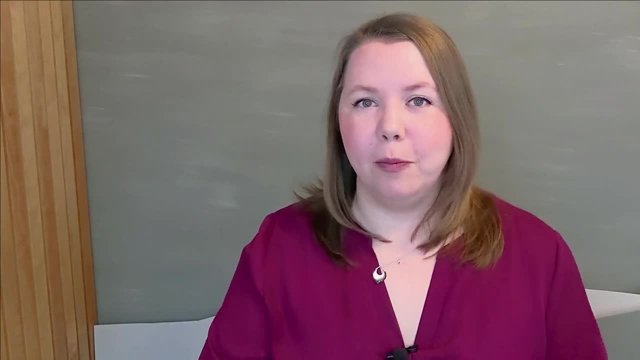 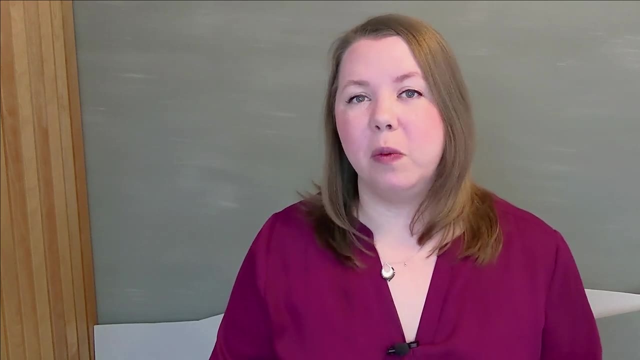 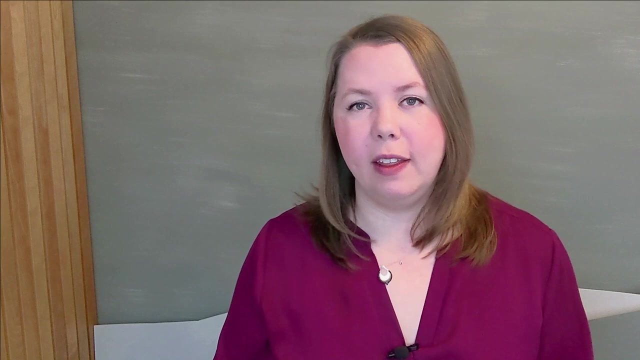 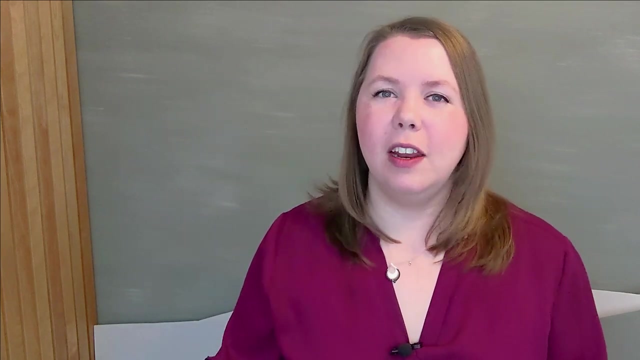 having direct interaction with patients that are being treated for a variety of health-related ailments or preventative care. these types of analysts often work with clinical data to help improve patient outcomes, and they also analyze patient data much in the same way that an analyst in any other field would analyze just general data for the company. the data may be specific. 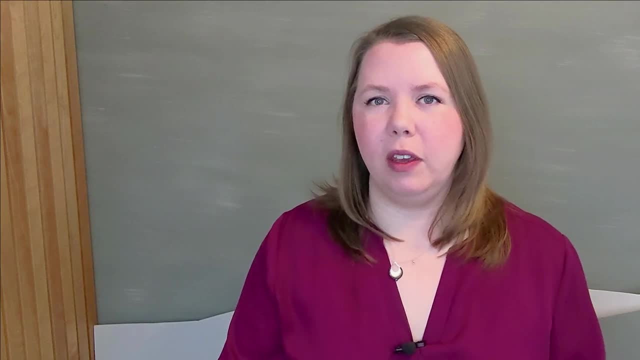 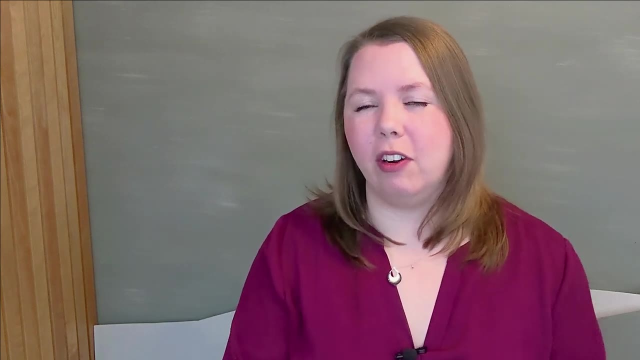 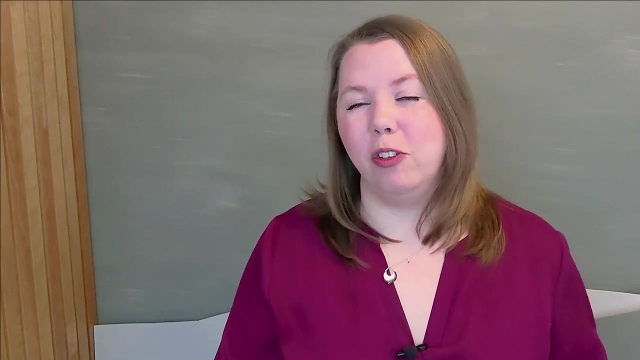 to healthcare, but a lot of the systems and information that's being used is quite reminiscent of customer data that's held in other fields. tools that manage electronic health records, or EHRs, are quite similar to CRM or customer relationship management software like salesforce, for instance, in a non-health setting. the second type of health care is the data management software. the second type of health care is the data management software. the second type of health care is the data management software. healthcare data analysts are ones that work for suppliers. suppliers cover a wide range of ground. some suppliers are software in nature, focused on, often electronic health records of patients. 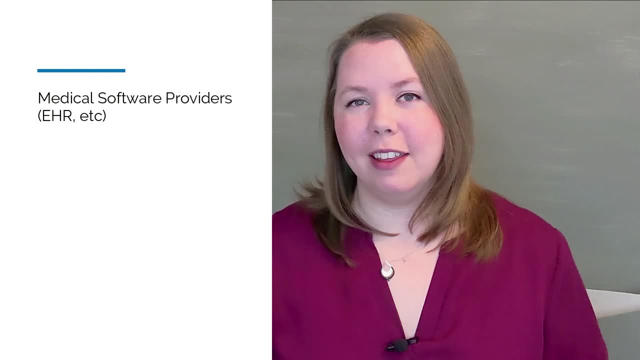 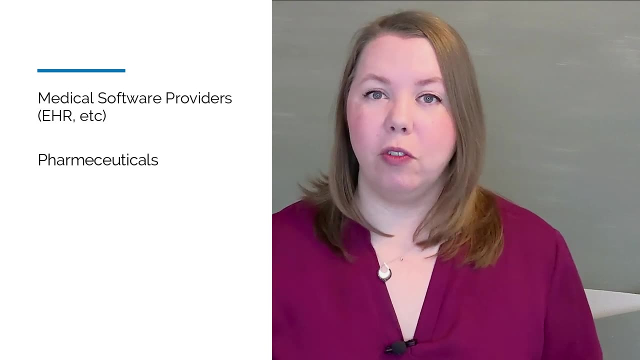 in tracking and even potentially analyzing the data that's collected there. suppliers also involve the pharmaceutical industry- companies that are developing pharmaceutical drugs to aid in the prevention or cure of different diseases- and it also involves device makers. medical supply companies also fall into this category, and these could 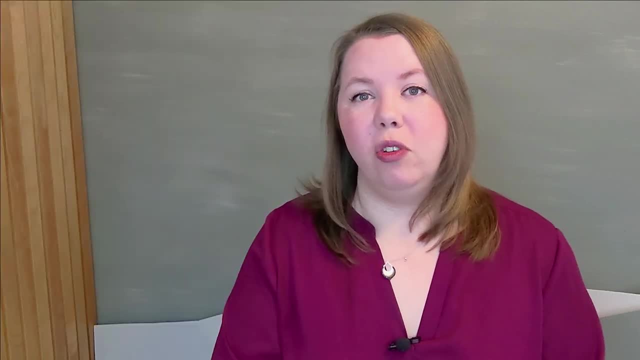 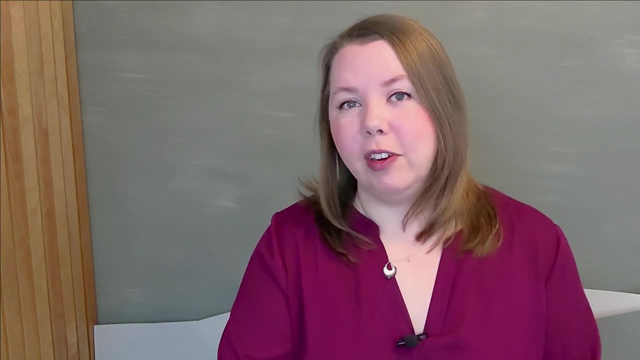 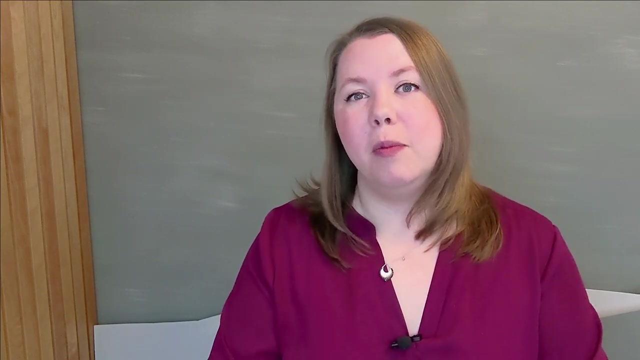 range everything from an implanted device to diabetic testing strips to bandages. anything that could be used in the treatment of any health related issue or prevention would fall into this category. the supplier category is probably the broadest because there are so many different niches where companies can work in a variety of different areas and they can work in a variety of. 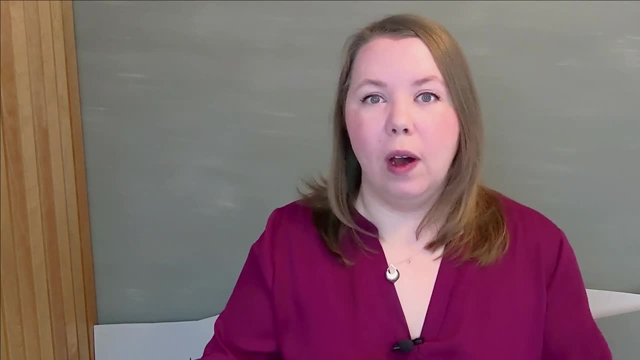 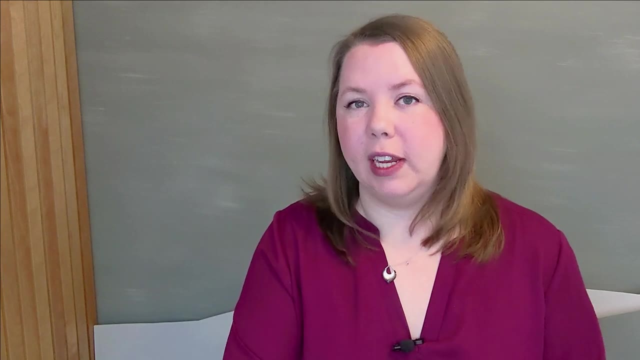 areas and they can work in a variety of different areas and they can work. and that's really going to and that's really going to determine what analysts- healthcare analysts- in that field do. in general, there tends to be a lot of focus on clinical data here, especially in the pharmaceutical 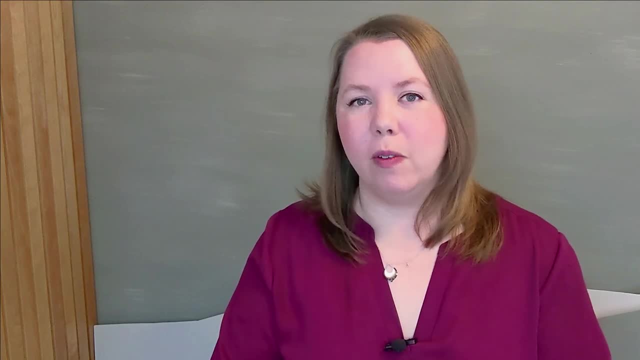 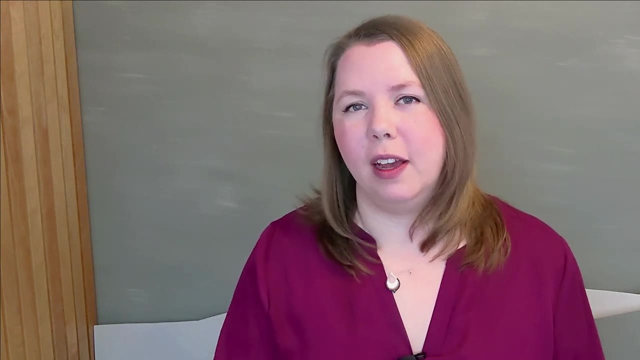 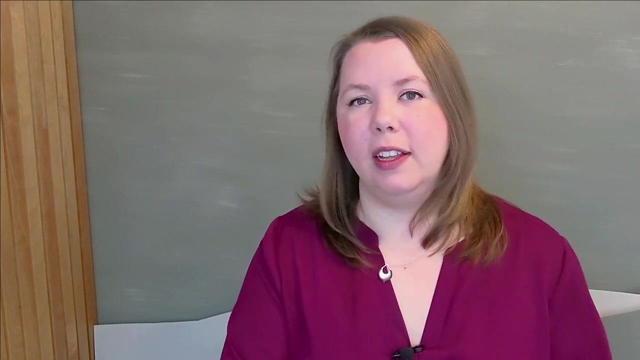 direction, but there's also a lot of application similar to other roles: tracking supply and demand, collecting data for improvement and using data to recommend new products or help design new products. clinical data analysts fall within this category and they use healthcare analysts analytics primarily to evaluate the performance of potential new drugs, to model drug interactions. 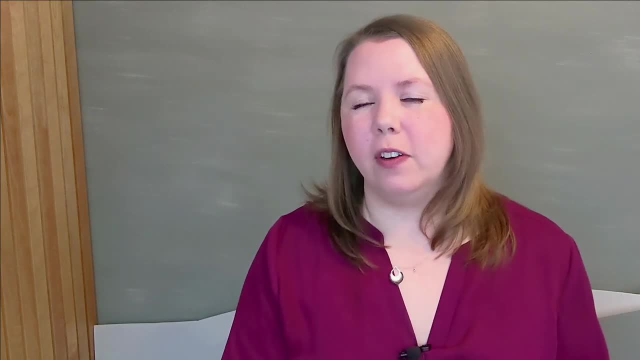 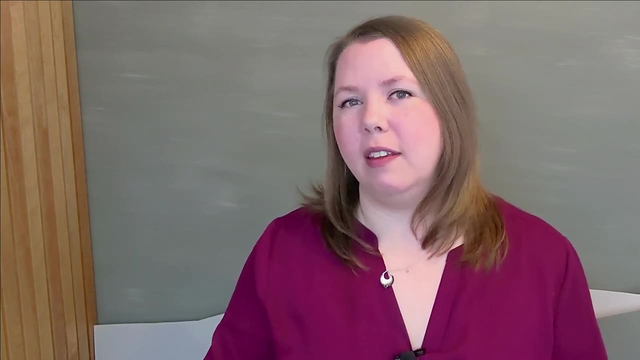 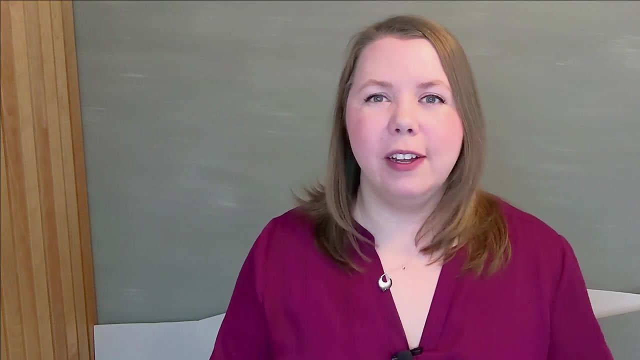 and so much more. these roles tend to be quite a bit different from a lot of other healthcare data analyst roles, which rely on much of the same techniques and methods and even skill knowledge that are used across all different sorts of industries. i'm going to talk next week, just 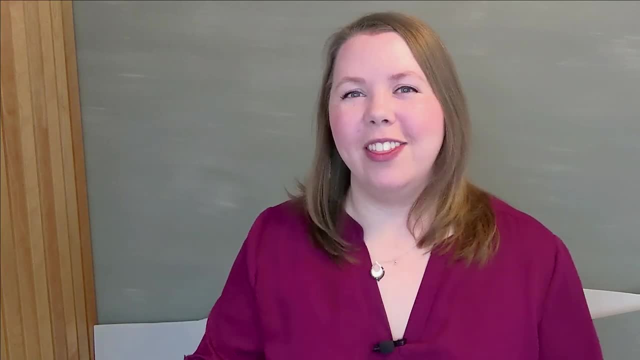 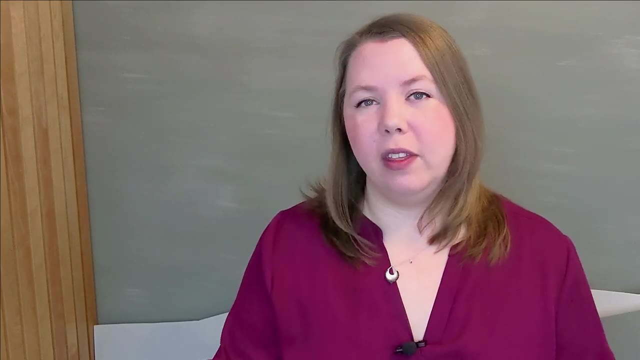 about clinical data analysts, because there's a lot to talk about here. type of healthcare data analysts are ones working in insurance industries. these are much more prevalent within the us than they are within a lot of other countries. simply because of the structure of healthcare, how it's provided and how it's funded, healthcare analysts in these roles can 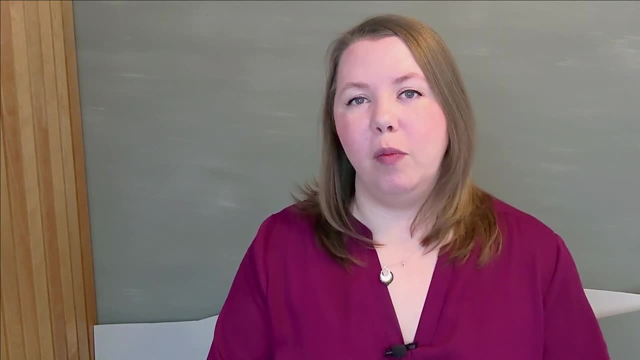 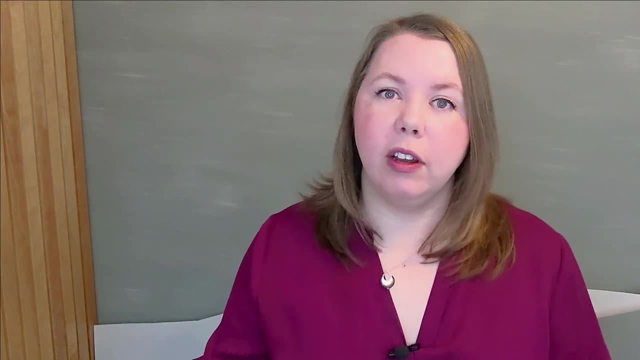 look at a variety of different data, everything from general trends about what the population that is insured may be experiencing- increasing or decreasing. specific health concerns that people are experiencing. increasing or decreasing. specific health concerns that people are experiencing- increasing or decreasing specific health concerns that people are experiencing, and they can also. 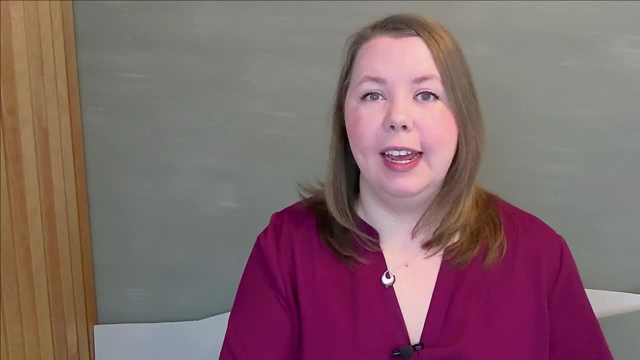 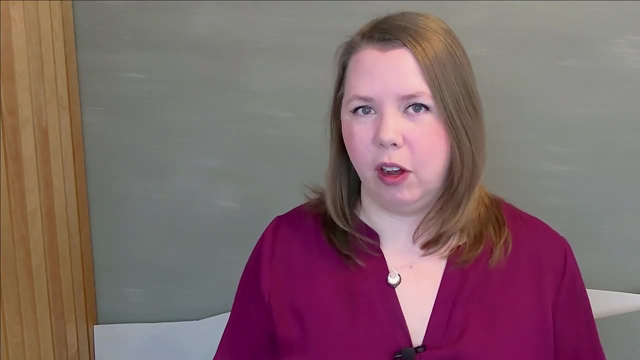 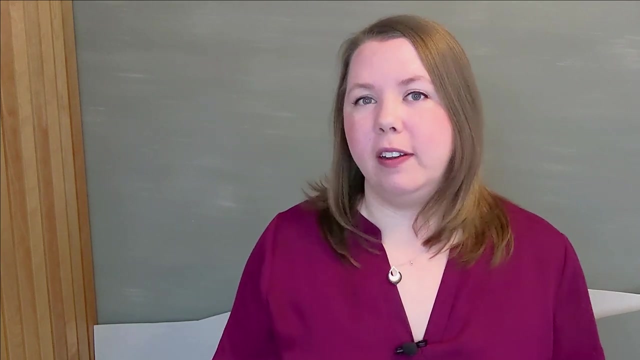 analyze very specific individual patient health risks and visits. ultimately, insurance companies are looking to minimize their expenses and reduce the cost of treatment. sometimes this aligns with the best interests of a patient, for instance, when they are able to recommend preventative measures that you can take to prevent health concerns down the road. on the other side, though, sometimes these interests are not aligned. what's in the best interest of the patient? perhaps experimental treatment or more expensive treatment- is not in the best interest of the insurance company's bottom line. it costs them more, and a more expensive patient to insure means that they're not making as much. i'm not going to dig into the pros and cons of the industry as a whole. 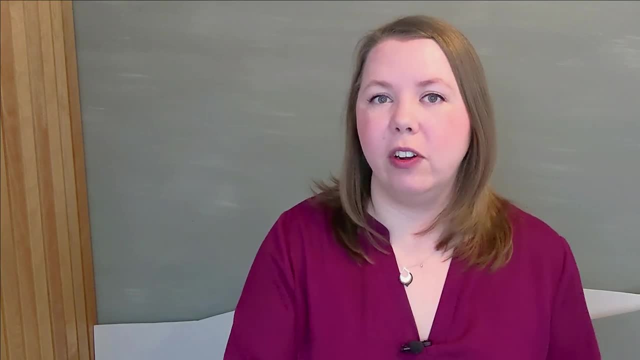 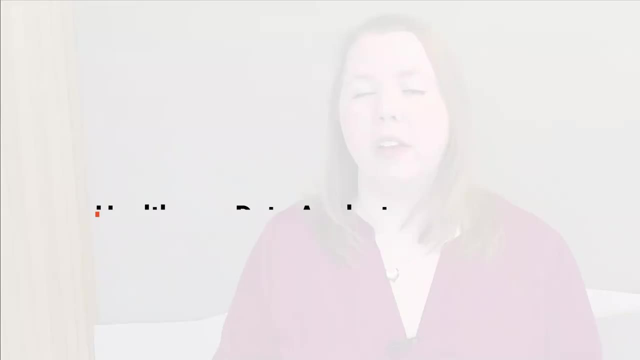 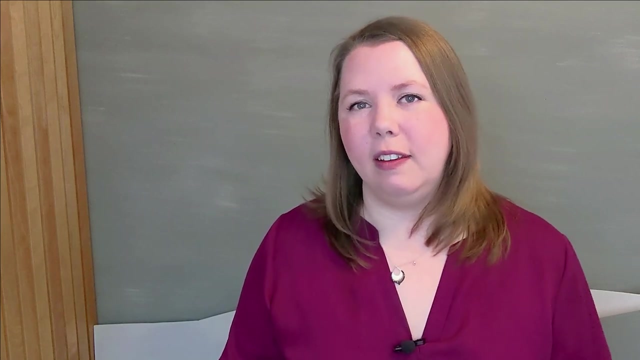 but i wanted to highlight the opportunity of healthcare data analysts working in this field. that brings us to the last major group of healthcare analysts, which are those that are working for policy or regulatory health care data analysts, and that's healthcare data analysts and that's regulatory organizations at a federal level. in the us, this would be organizations like the cdc or the. 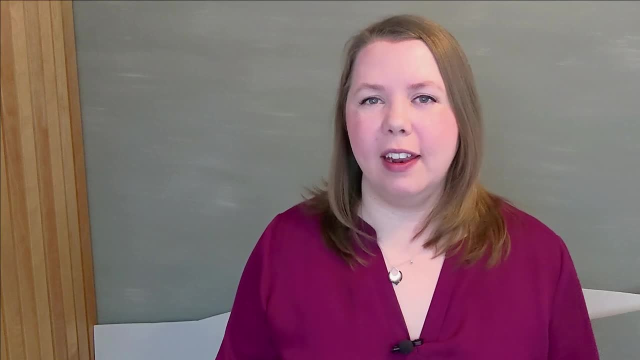 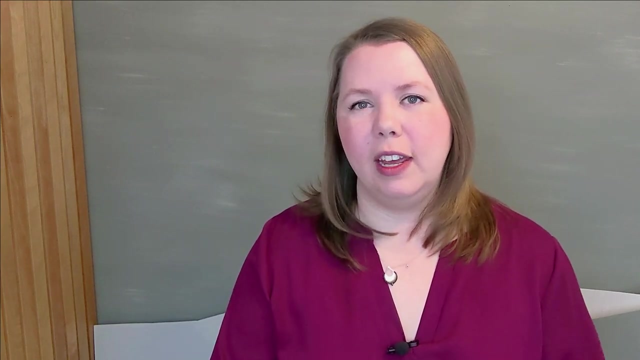 fda in canada. it might be statistics canada, but it's also often prevalent in state or provincial governments that are looking to track performance, analyze performance within their certain area. these roles typically concern themselves with understanding the complete picture of public health within whatever area of coverage that they have their work. 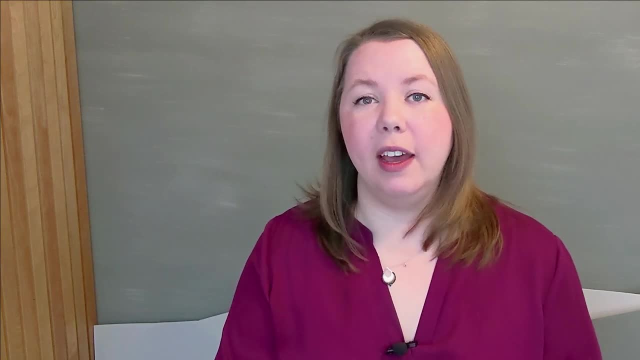 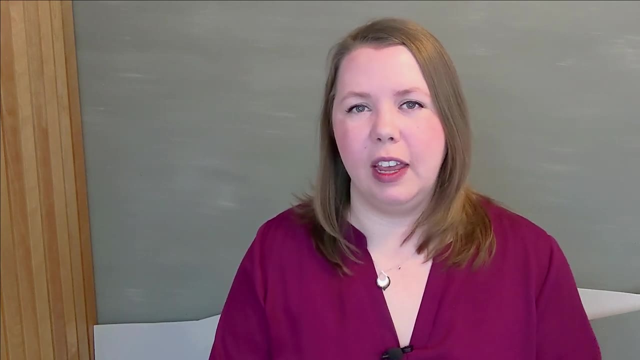 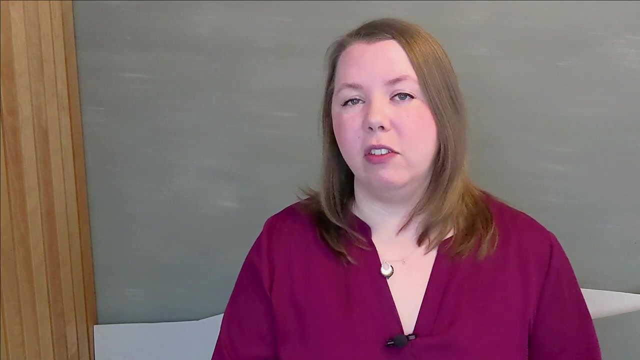 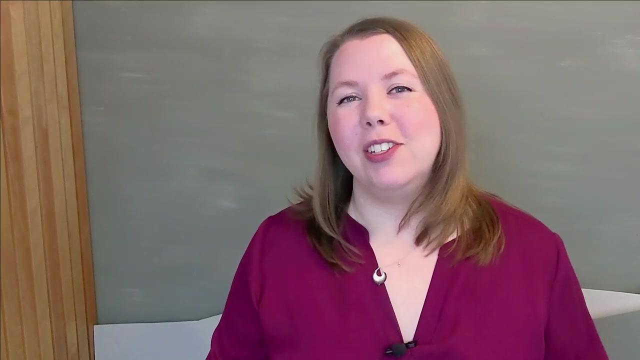 often factors into public health programs and hospital or provider ratings. from this work we learn what health concerns are increasing or decreasing and what populations are perhaps most at risk of different conditions or have been experiencing certain conditions more than others. i mentioned that these are broad titles and the titles aren't completely uniform while i talk. 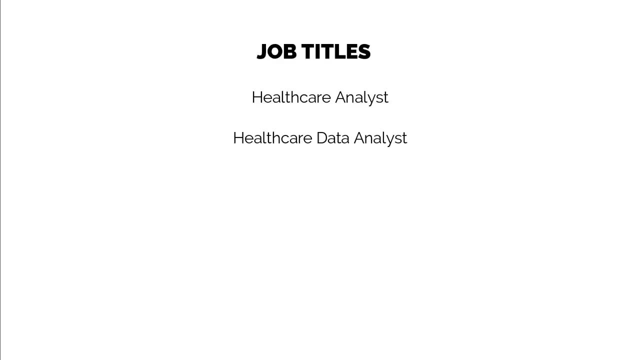 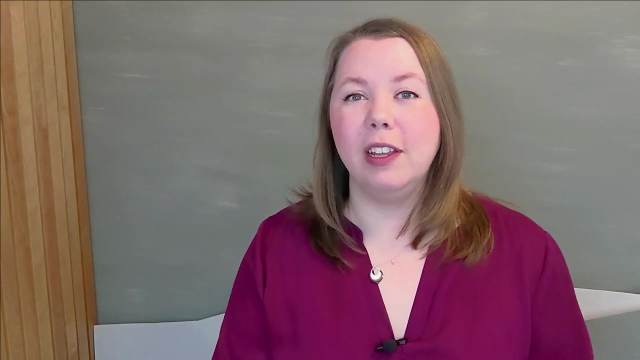 about the role as a healthcare data analyst. you've also heard me mention healthcare analysts throughout the video and similar roles, depending on the niche, could be called health information management analysts or him analysts, healthcare business analysts, electronic health records analysts or ehr analysts, or even statistician, depending on the role. a major question that often arises. 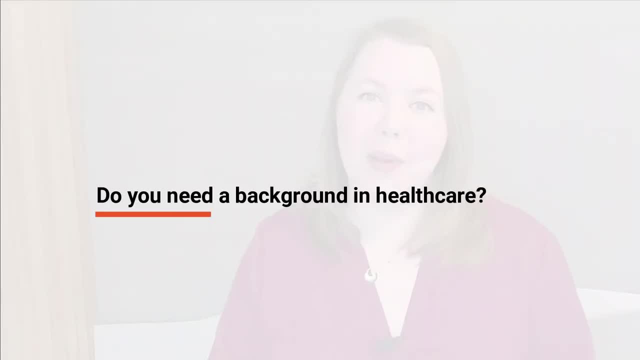 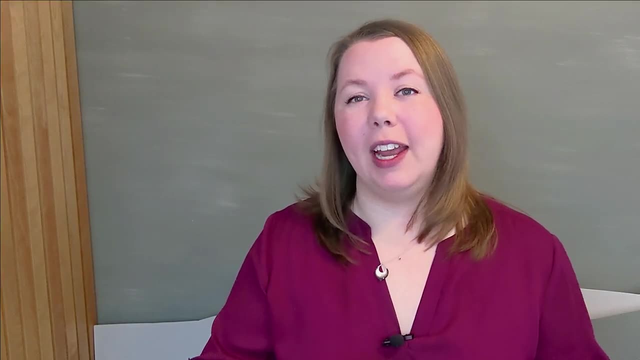 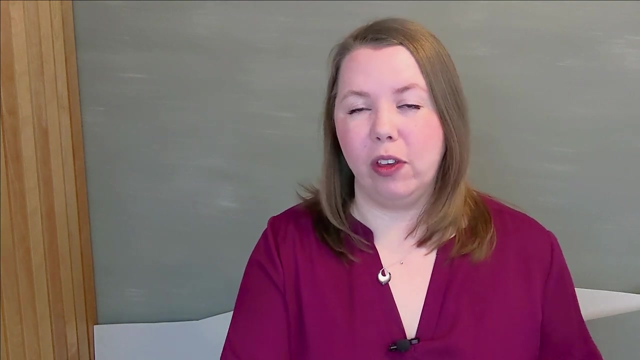 in relation to healthcare data analyst roles is: do you need a background in healthcare to get into one of these roles? a lot of this is going to depend on the specific area that you're working in, like any other field, having some knowledge that's specific to healthcare or healthcare supply or whatever the area that you're focusing on, of course, having 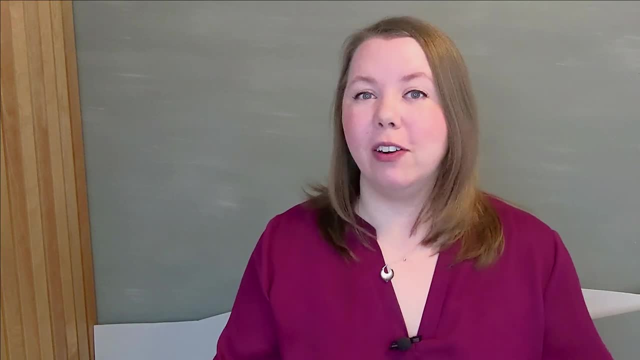 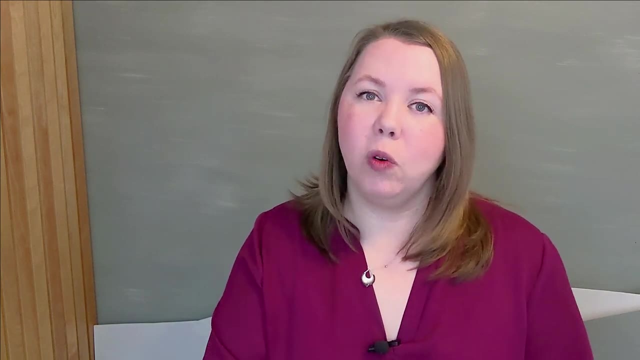 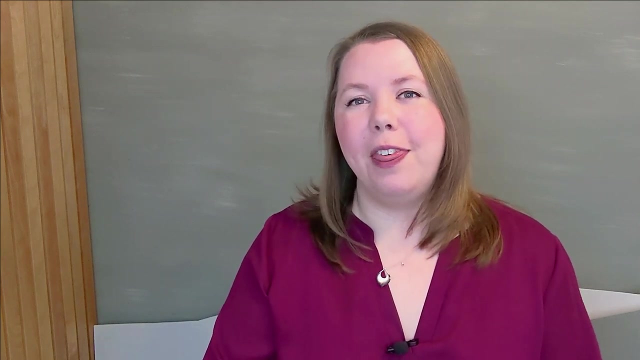 knowledge in this area gives you an advantage. it's subject matter expertise, and any company tends to benefit from people that have this sort of knowledge. in some roles it's going to be less critical than others. for instance, if you're working for a supplier of steel or proceed to a point where there is a shortage of resources, you're more likely to 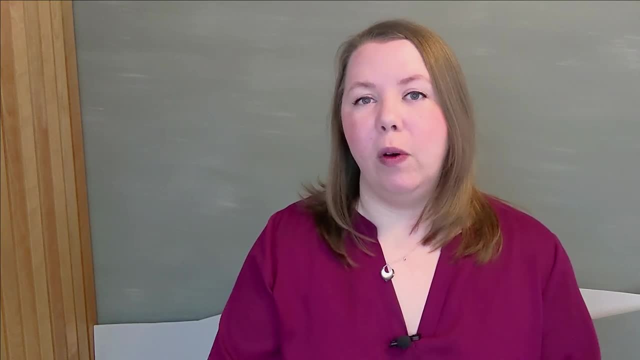 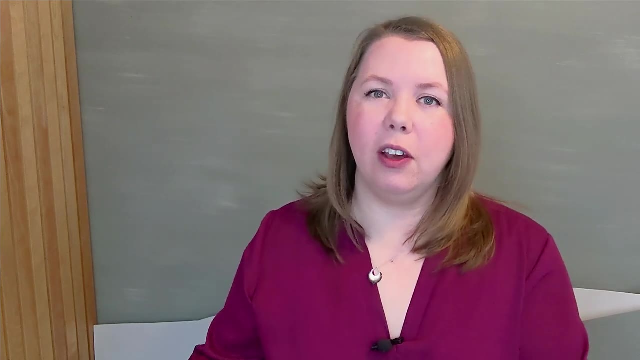 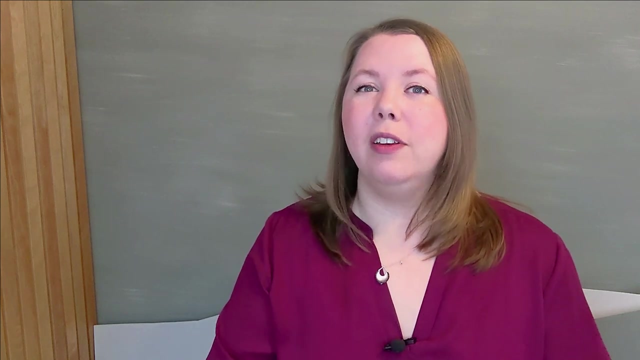 have a balance of content because you don't have a lot of persons or work at a or your department, government or the history department or other infrastructure department. Eating candles is a fabulous number as an award for healthcare. you have the option of having an award for trying something or the other, a company that like an award or a company that